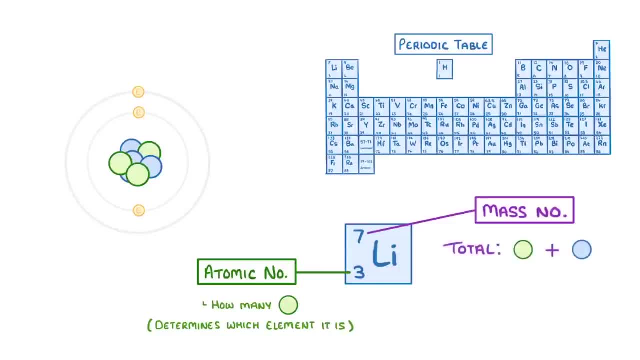 In the top left we have the mass number, which tells us the total number of protons and neutrons together. So lithium's is 7, because it has 3 protons and 4 neutrons, And this one's really important because it's the number of protons that determines which. 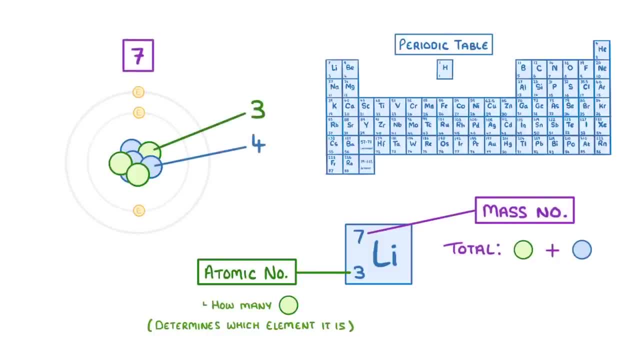 element it is. So lithium's is 7, because it's the number of protons and 4 neutrons which together makes 7.. Now, the nucleus symbol doesn't directly tell you the number of electrons. You just have to remember that the number of protons and electrons in an atom is the same, which is 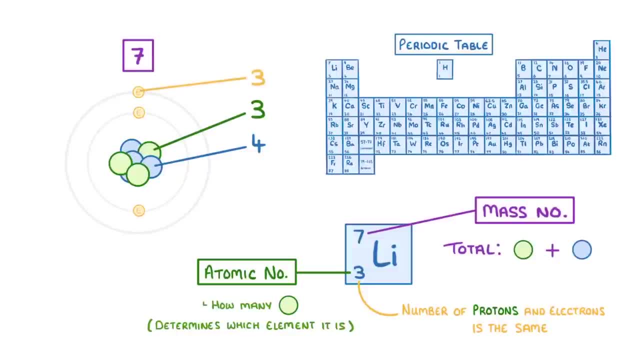 why lithium has 3 electrons. The next thing we need to look at are isotopes. The isotopes of an element are atoms with the same number of protons and neutrons. Lithium's is a bunch of electrons, so the same atomic number, but different numbers. 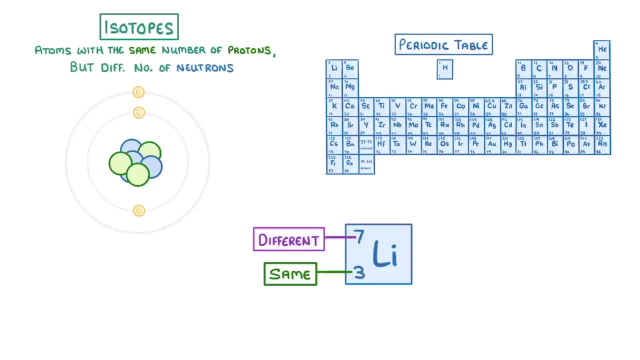 of neutrons, so different mass numbers. For example, as well as lithium-7,, which we've been looking at so far, we can also get lithium-6,, which has 3 neutrons, and lithium-8,, which has 5.. 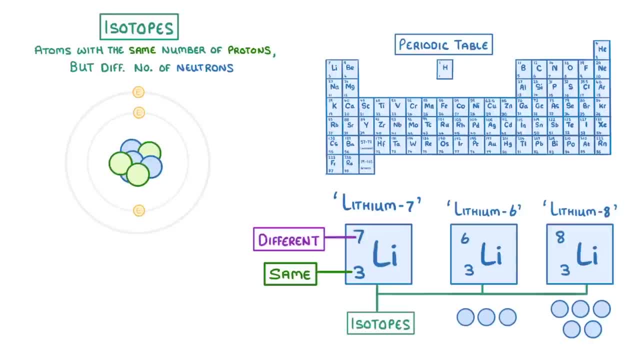 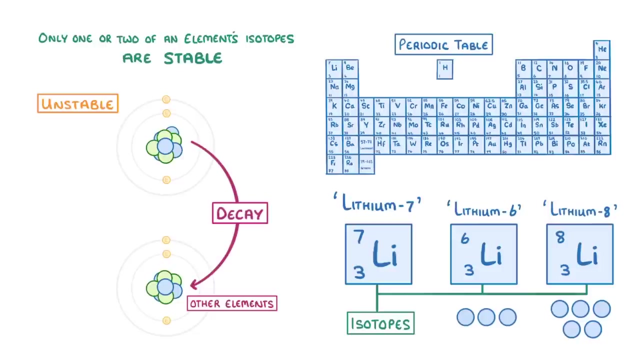 So these three would all be classed as isotopes of lithium, because they all have the same number of protons but different numbers of neutrons. Now, generally, only one or two of an element's isotopes are actually stable. The other isotopes, which are unstable, tend to decay into other elements by emitting radiation. 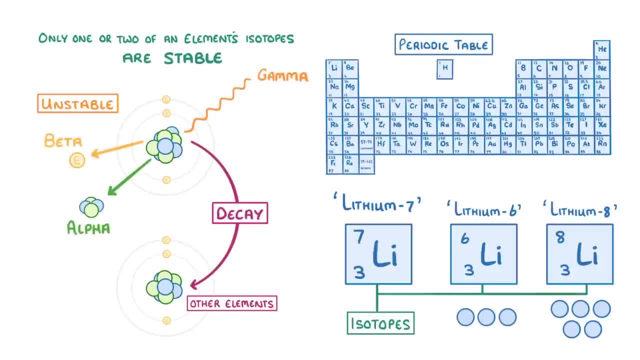 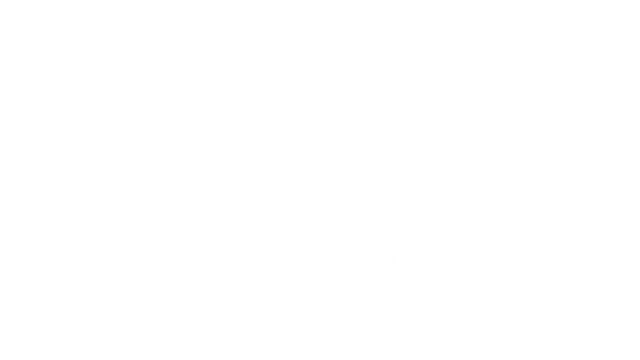 like alpha, beta or gamma radiation, or sometimes they just emit neutrons. We call this process radioactive decay, and we'll take a closer look at it in the next video. For now, though, we need to take a closer look at the electrons. 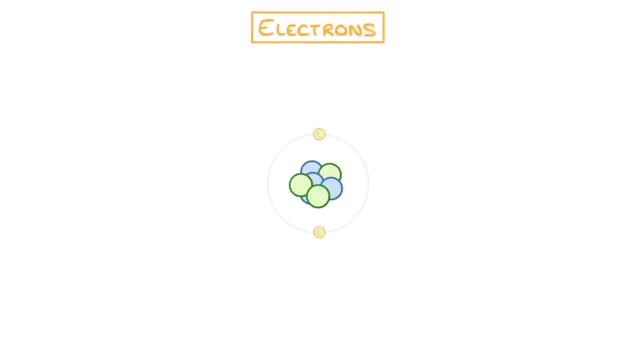 The electrons in an atom are arranged in a series of energy levels, which we call shells, with each shell getting progressively further away from the nucleus and increasing in energy level. Although electrons normally stick to a single shell, as they always do, they tend to be. 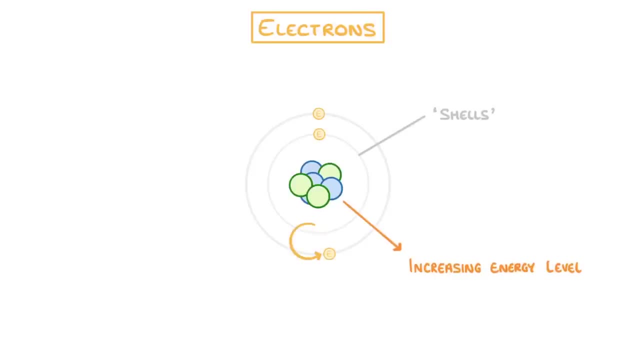 more at the nucleus. They can occasionally jump up to a higher energy level if they gain enough energy, and at that point we'd say that the electron has become excited. The energy for this comes from electromagnetic radiation, and it will only work if the radiation